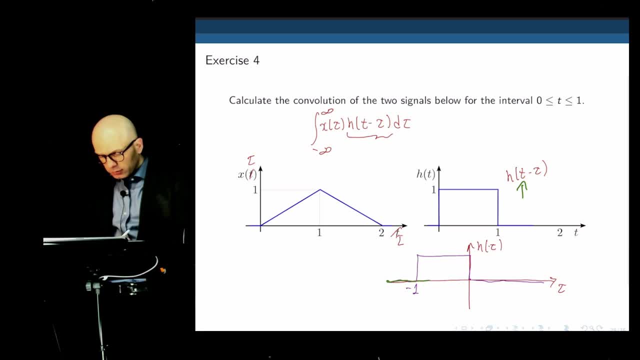 as we see in there, we shift the entire function by a amount of T. So if that's T, this here is T minus one. Why T minus one? Because the width of that is one Right. So are there any questions? up to this point, 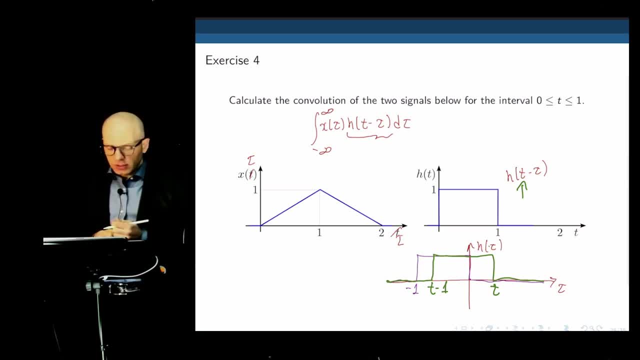 That's how we conversed the function H of T into the function H of T minus tau. Now, yeah, okay, Why isn't T minus one all the way back there on the purple line, On the purple one? which one's purple? 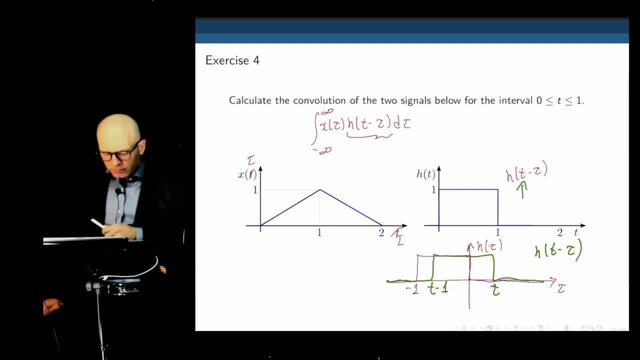 For the T minus one. I'm just trying to wrap my head around it. Yeah, Yes, so if we just flip the, the, the graph, that's what do we get. Are we okay with this? Yeah, Yeah, So now if we add T to the entire function, the whole thing shifts, So zero becomes. 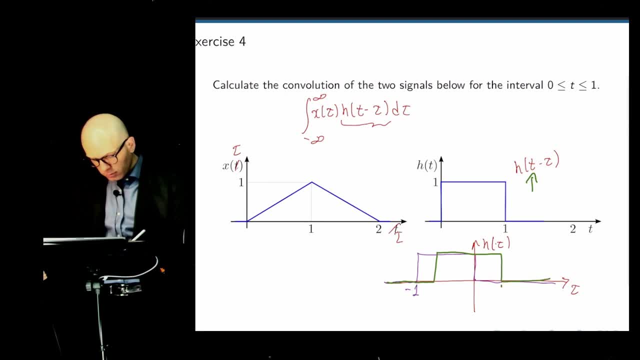 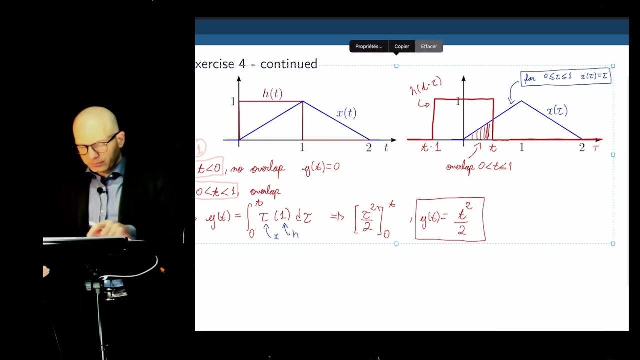 T, Right, Okay, And the back here becomes T minus one. So this width is still one. This width is still one. It's a time shift, right, You are not stretching your mouth. If we are multiplying, that would increase the way. Okay, Thank you. So that's, then the expression we have. Let me erase this. 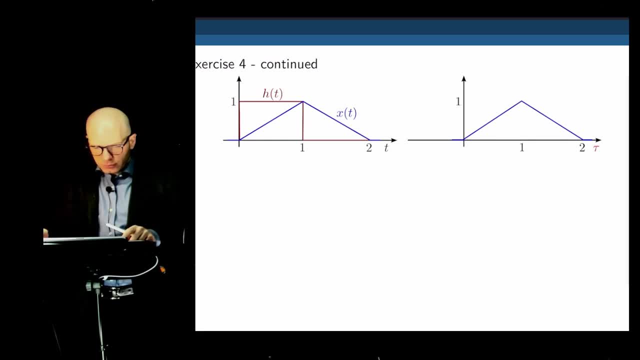 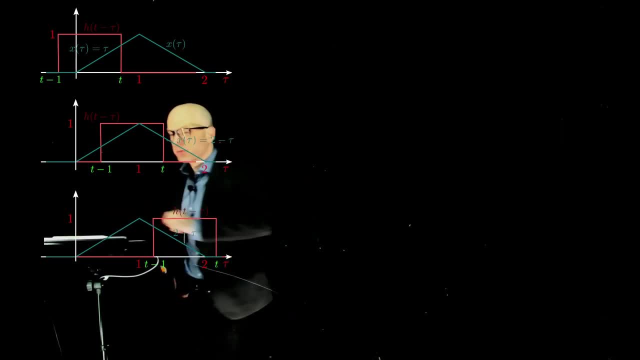 And what do we do next? Well, uh, actually, let me move to the light board, What we'll do next. So here we have the expressions We the, the graphs we derived. So this is the T, T minus one that we just flipped, that is H of T, And this is the other expression. 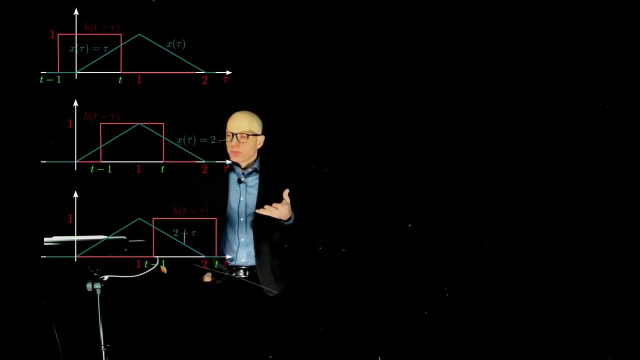 the other graph. Now, when you take the integral, that integral has a value of T inside that is unspecified, which means that if you're not looking at the entire tau axis, that value of T needs to translate, needs to cover the entire tau axis from negative infinity all the way to. 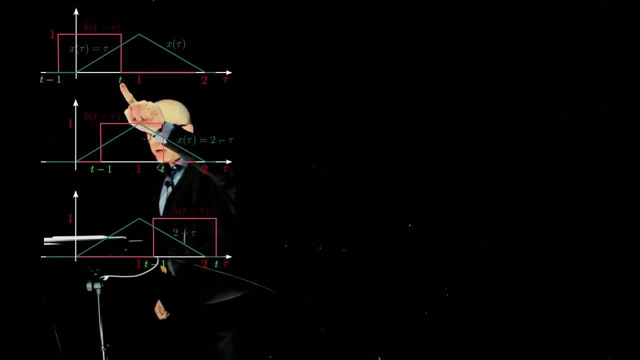 positive infinity. So now I have to take this value of tau and make it move along- excuse me, the value of T And make that move along the tau axis, And then look at our overlaps between just two functions, that we are taking the convolution out And by covering out the entire tau axis. 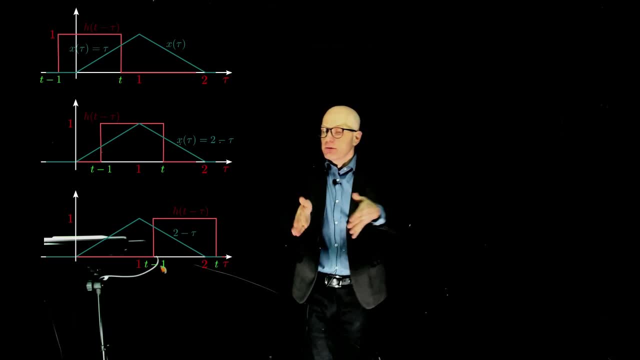 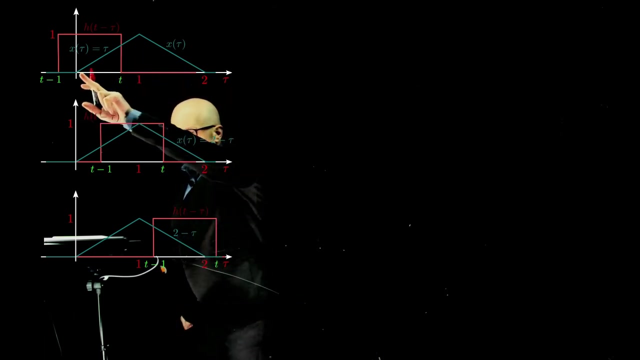 we look at different portions that have different overlaps and then you perform the integration there. So one thing to note here is this triangle. So you have two parts of this triangle Now this one here is a ramp that starts from zero and goes to one at time, one. 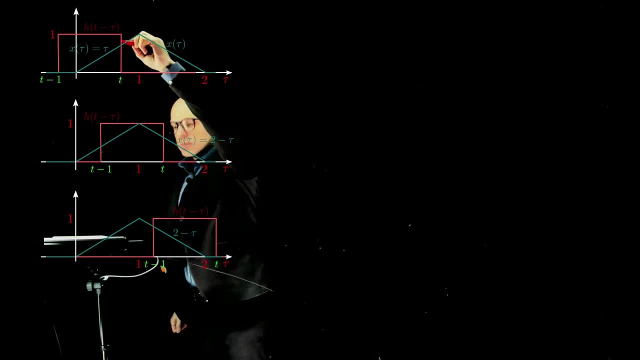 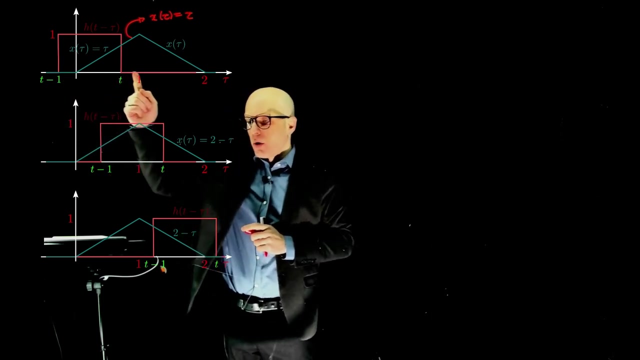 So we can say that for this part, H of tau or X of tau is simply equal to tau, And this is only valid between zero and one right. When tau is one, H of tau is one. When tau is 0.5, H of tau is 0.5. 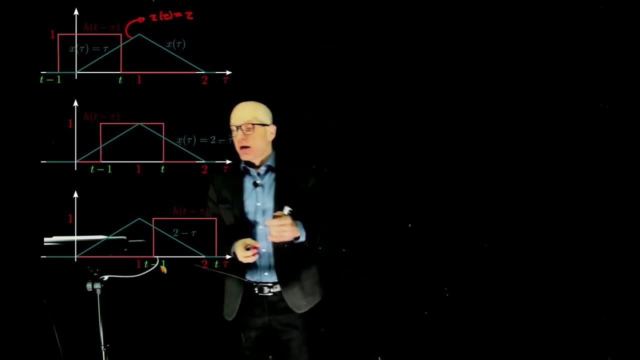 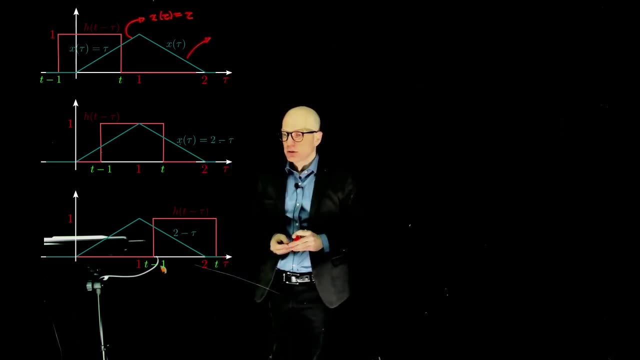 So for the first time past one that relation has changed And that a curve here between one and two is a bit different. This is still a linear curve, but you can say now that X of tau is two minus tau. Let's verify that when tau equals to one, the value of the function is one. 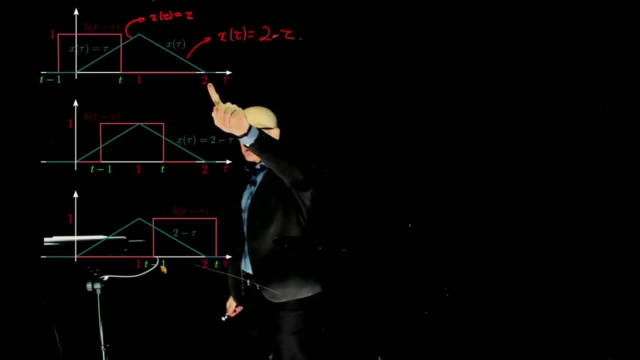 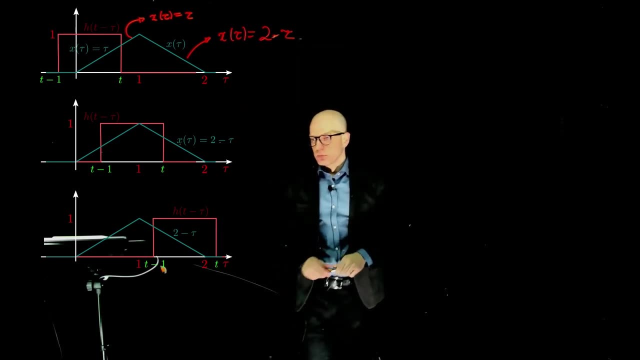 So two minus one equals to one. that holds, And when tau is two, the function is at zero. tau of two equals to two minus two. that's zero. okay, So now we have all the expressions we need to integrate. We have the expression from zero to one for this curve. 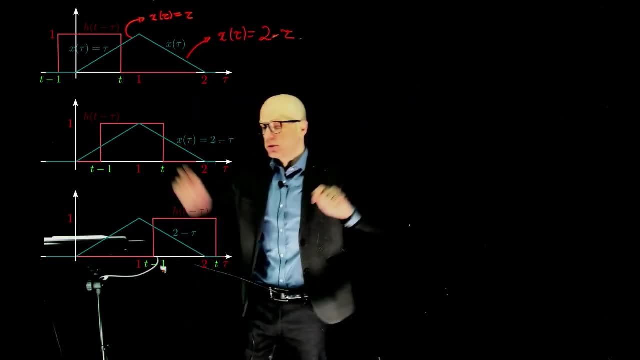 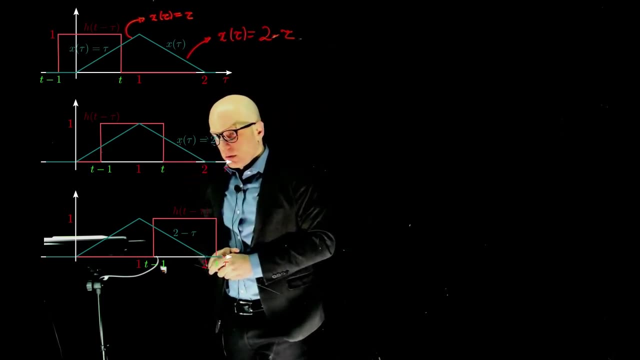 and from one to two for that. And you know that a pass two, it's zero, Lower than one than zero, it's also zero. What is next? Well, now we need to perform that integration, famous integration, which is the integral. 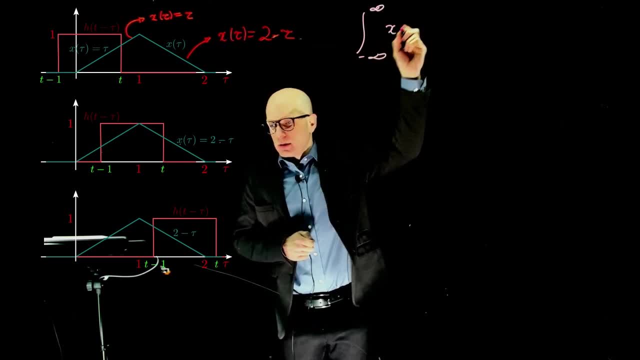 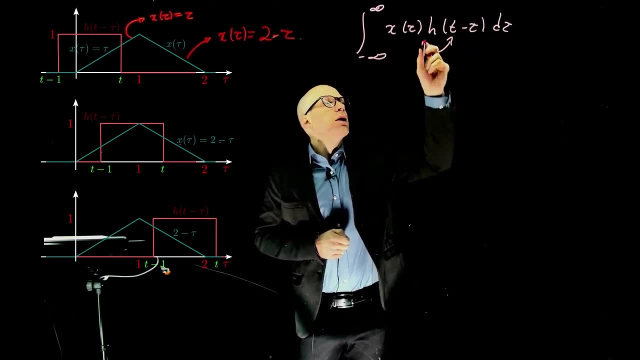 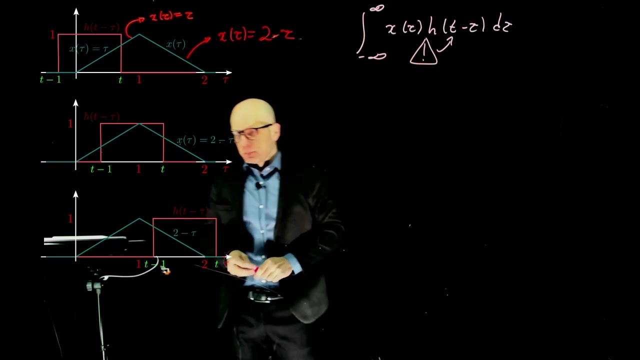 from negative infinity to infinity of X, of tau H, of T minus tau, D, tau. Now T here is unspecified, So T needs to now translate cover the entire tau axis. So let's just start with T going to negative or less than zero. 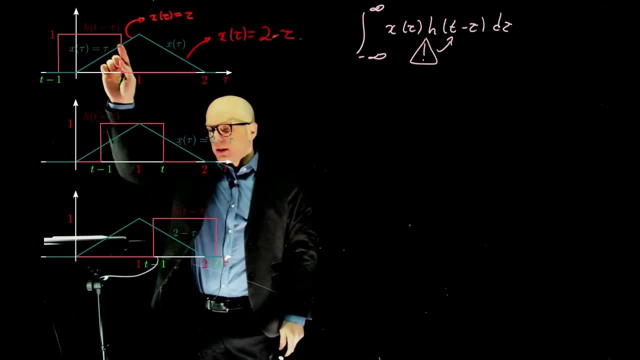 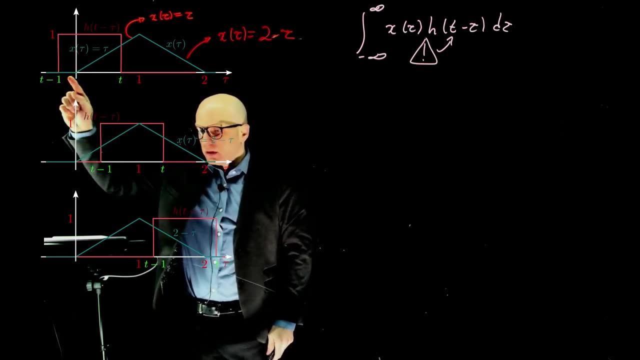 If T is less than zero, then this block will be up here, And when T is less than zero, we are multiplying zero with zero or with a function of tau. So provided that a T is smaller than zero, the overlap there is a function times zero. 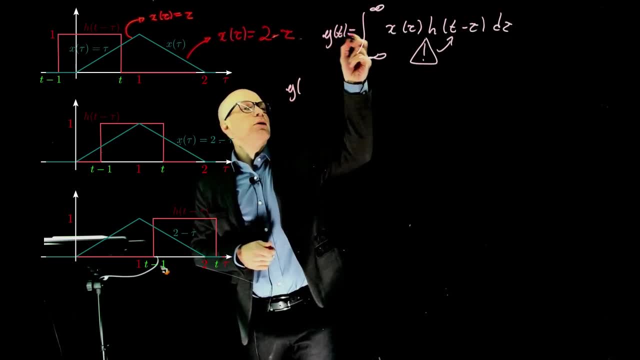 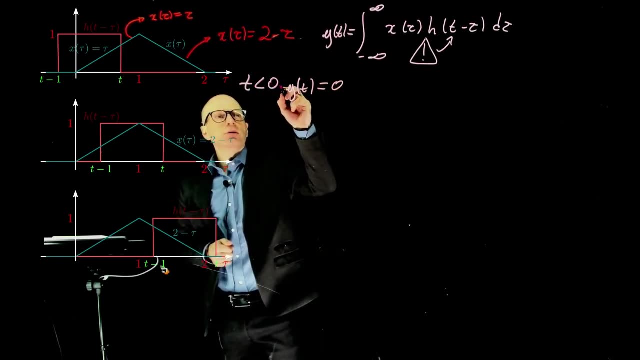 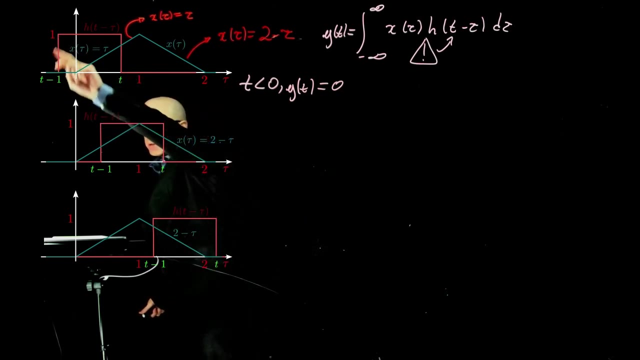 And the result of this integration- let's call this Y- of T is zero. So this is: for T is smaller than zero. I noticed that for T is smaller than zero Doesn't matter where this function is, because the other one is always zero. 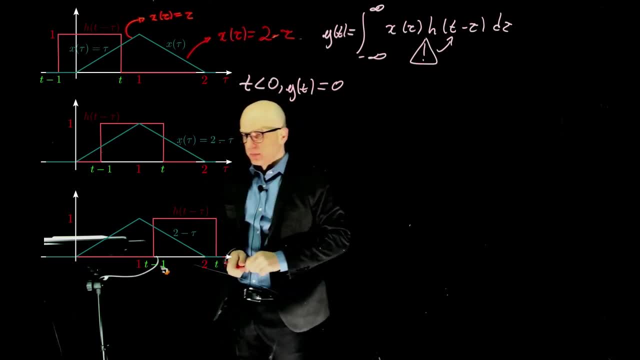 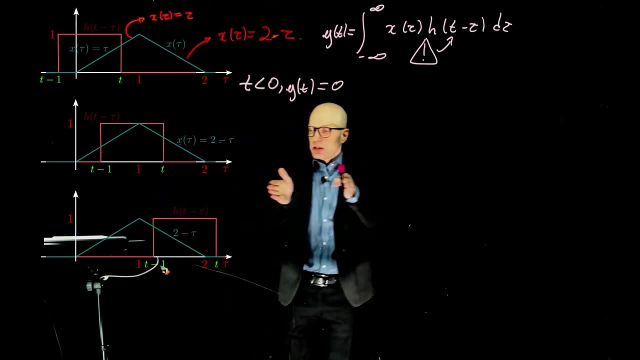 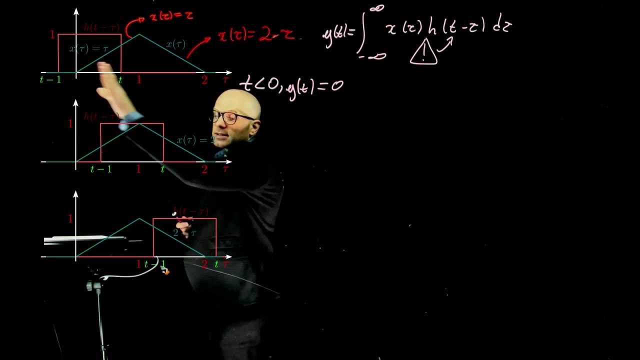 So when you multiply them, we get zero. Now let's, now that I covered the entire negative axis, we can start to translate T and move that towards the positive. So that's what we see here: T has entered the positive values. 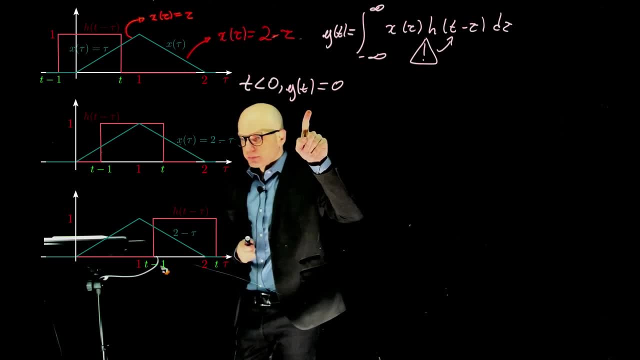 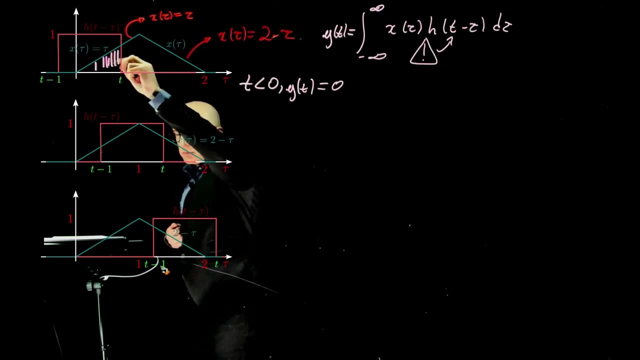 We are no longer in this region, here, And because you're no longer there, what can we see? Well, we see clearly that there is an overlap there of two non-zero functions, And that overlap will exist provided that a T is smaller than one. 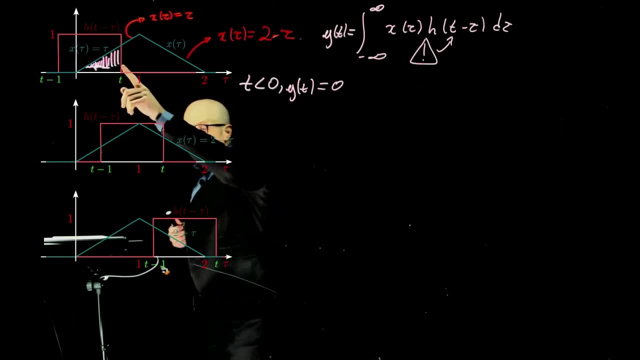 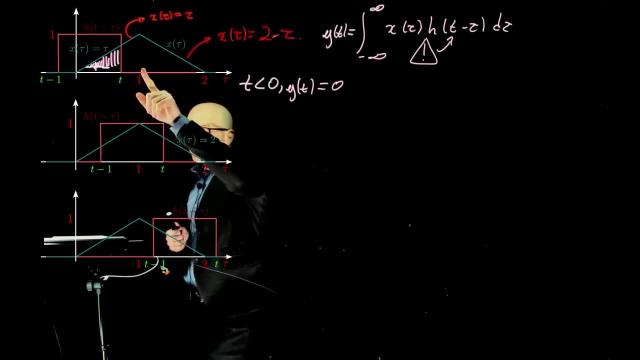 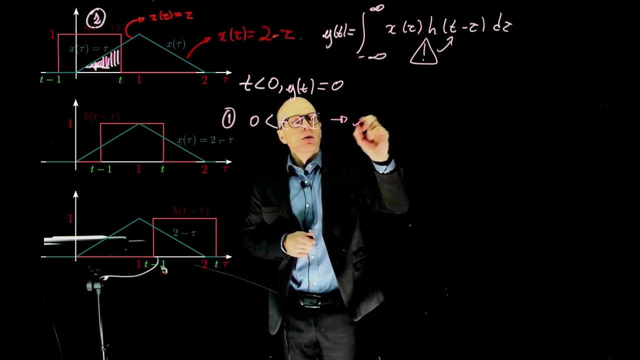 We need to account for that separately. So for this first part, if T is greater than zero, but it's smaller than one, here is the overlap, This is one Right, here is the overlap. And what is that overlap? Well, we can do the convolution there. 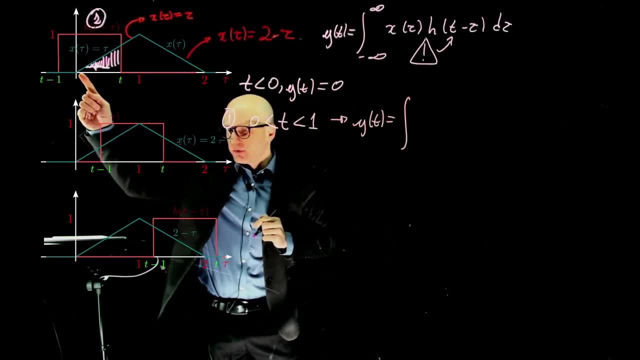 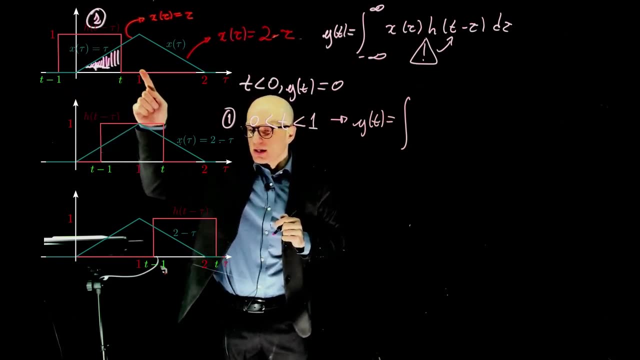 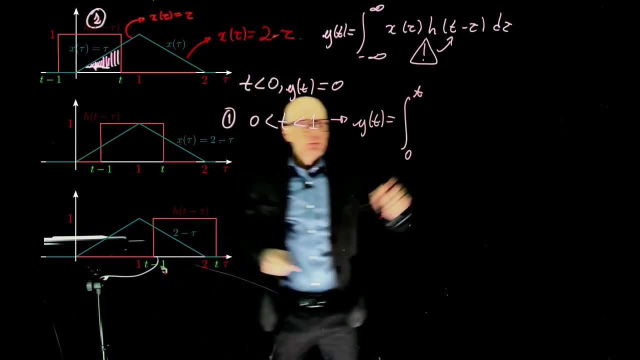 by taking the integral. that is only valid for the overlap. The overlap exists from zero to T right, But a T can only go as high as one, So the overlap exists from zero to T. X of tau. is this function which turns out to be tau? 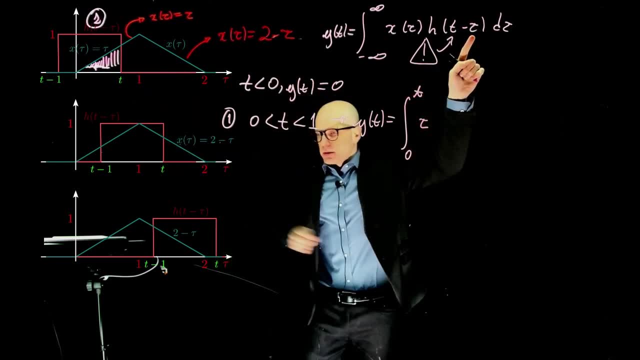 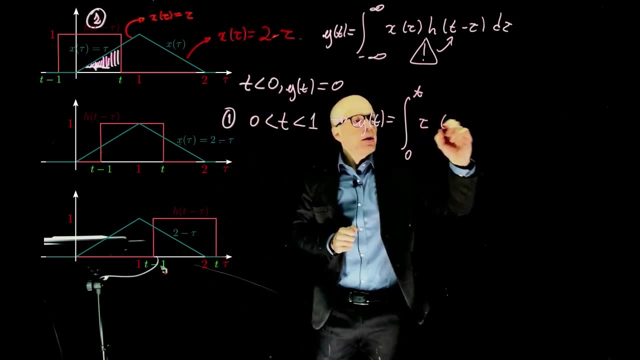 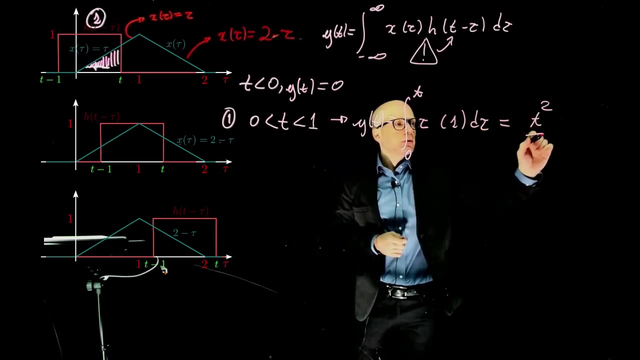 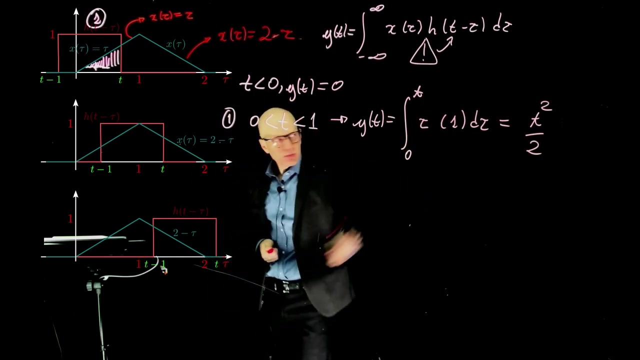 H of T minus tau is the red curve which in this interval is worth one d tau, And this integral gives T squared over two. My tau integral of tau is tau squared over two. Replace that T squared over two. Are we good with the first integration? 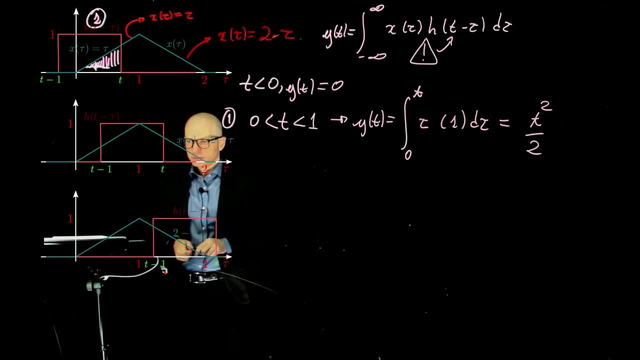 Sorry, could you just repeat why the limits of integration are zero to T instead of zero to one? Yeah, so I just wanted to point out that I am already out of like five minutes more than where I want it to be, but I'll continue. 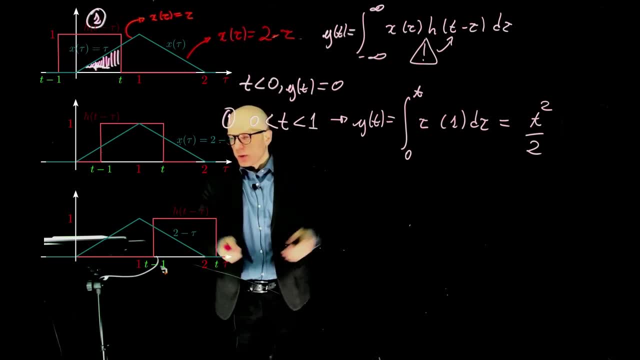 And so we have this in the record. And so if you have any other classes, any other commitments, feel free to leave. I will continue this and then post the solution. Yes, so do we agree that, at this interval exactly that, we're going to be able to do this? 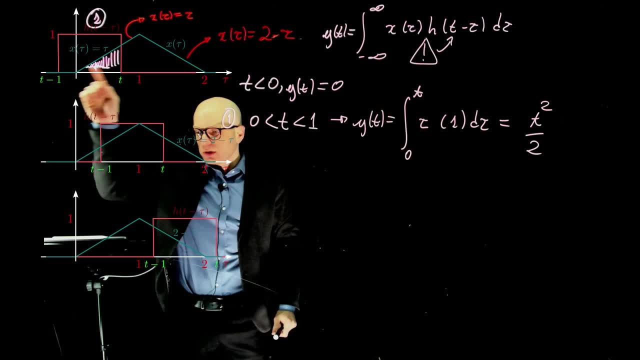 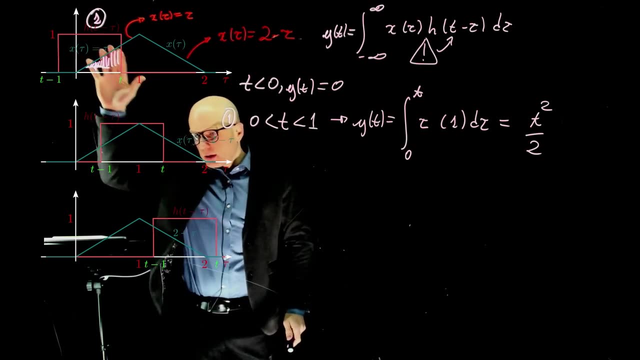 What is the interval exists between zero and one. This overlap between zero and one Right, so long as T is between zero and one. there exists an overlap there. But that overlap only exists between zero and T right. There is no overlap past T, because it's zero. 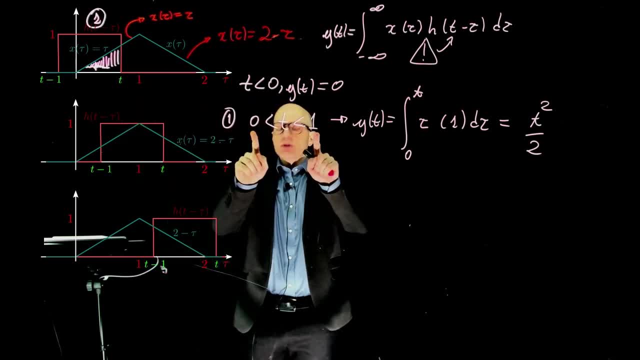 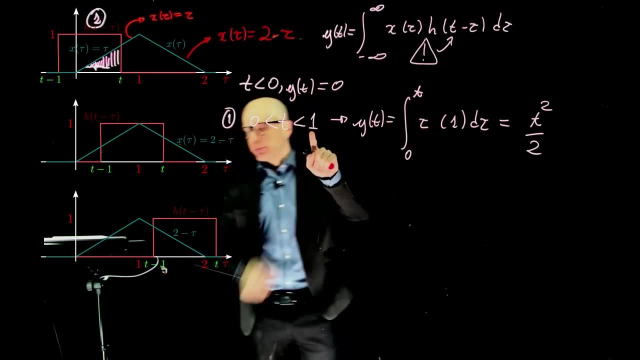 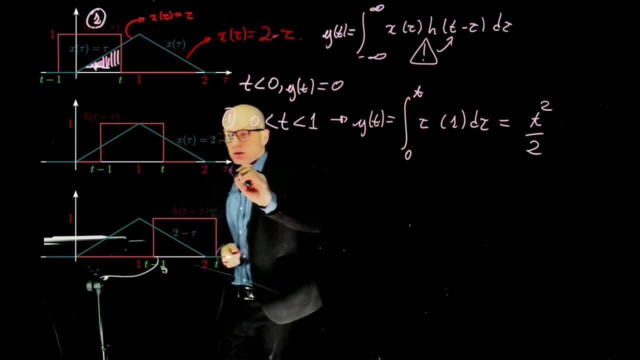 Oh right, yeah, yeah. So, even though we are considering this interval, we need to stop at T, but T may go up to one, right Up to one. Okay, yeah, I see now, Yeah, so now let's do this. 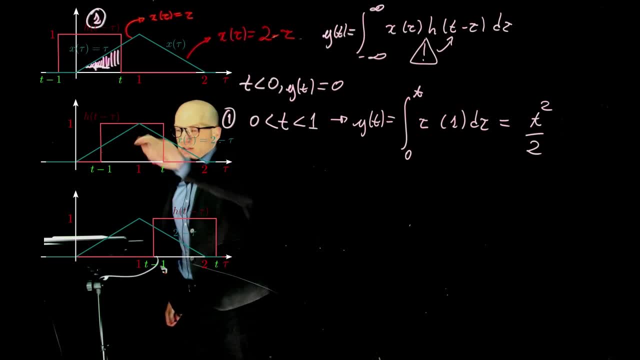 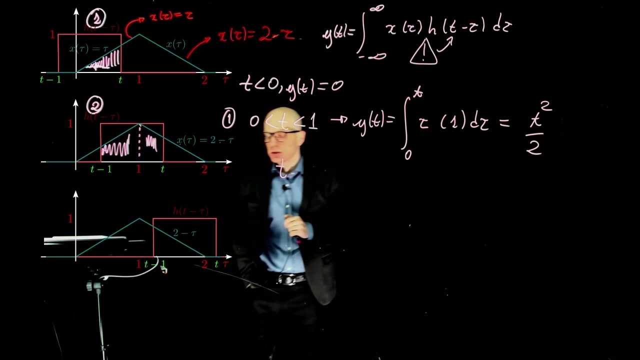 Now, when you pass one, which is the second graph here, we pass one, and we are now between which values? So long as T, we see two overlaps. right, We see one overlap here and you see another overlap there, So these are two distinct ones. 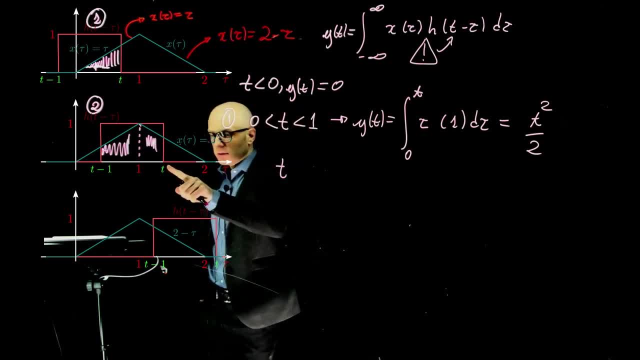 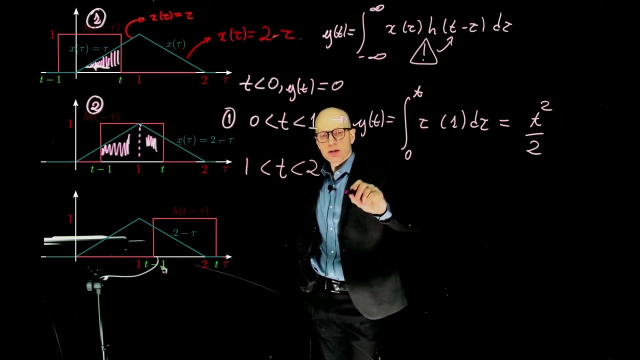 And this overlap will exist so long as T is between one and two. So long as T is between one and two, these two overlaps will exist. Yeah, So what is the integral there? Is this first one here, which is integral from. 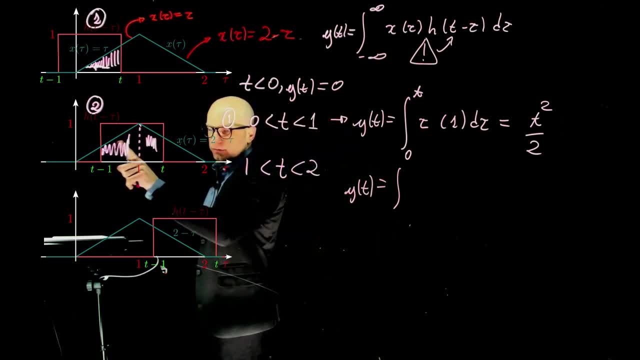 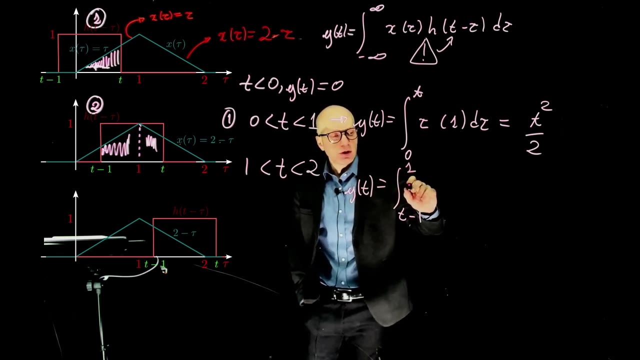 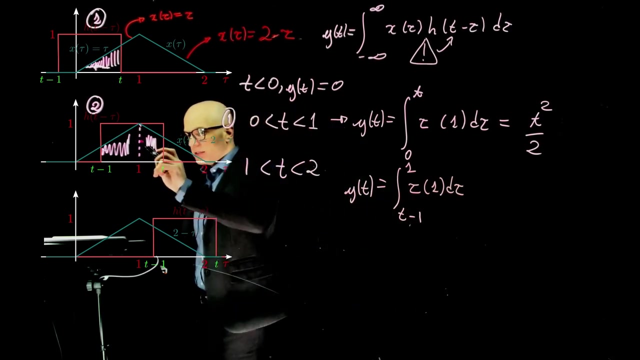 what is this limit? This first overlap, First overlap exists between T minus one and one, So T minus one and one of the two functions, which is tau times one, D, tau plus the second overlap here. The second overlap that now exists is between one and T. 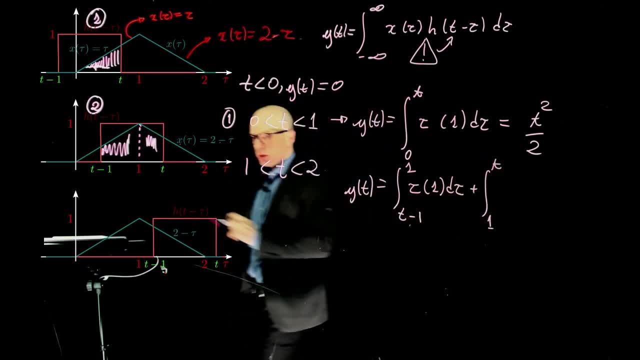 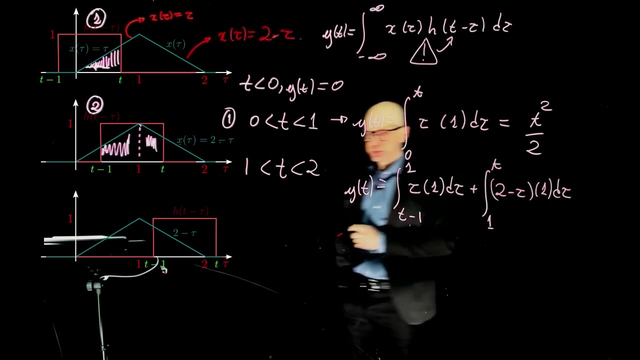 One and T. Now we are taking the overlap between is still X of T, which is one, but now this function has changed And this function is two minus tau times one D tau. So now we are taking the first overlap and this is the first overlap. 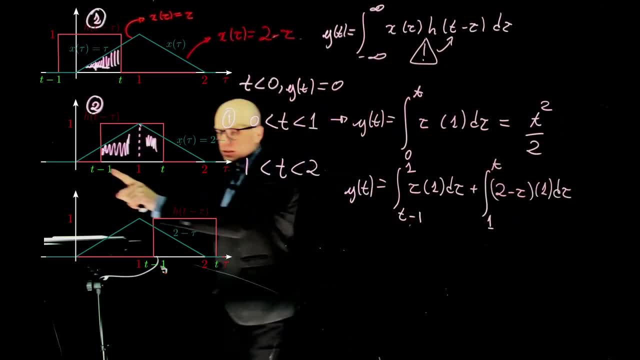 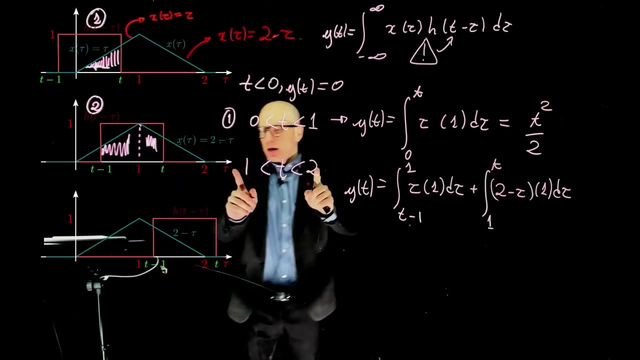 First overlap, Second overlap. First overlap exists between T minus one and one. second overlap exists between one and two, And this can occur so long as T is between one and two. Okay, Now we can move on If we pass two, and this is really, this is really. 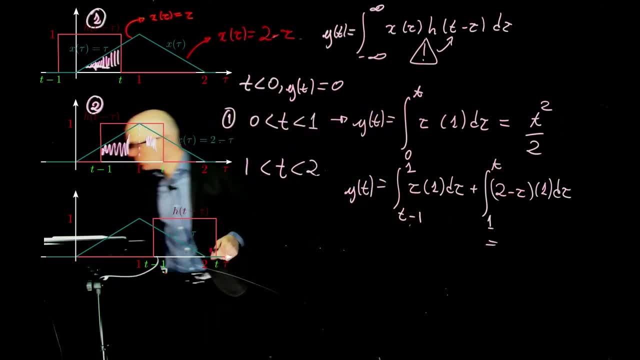 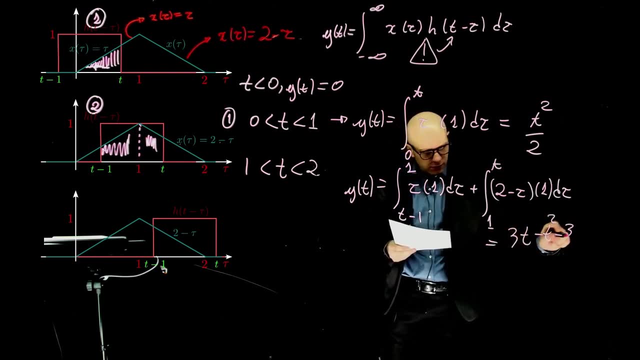 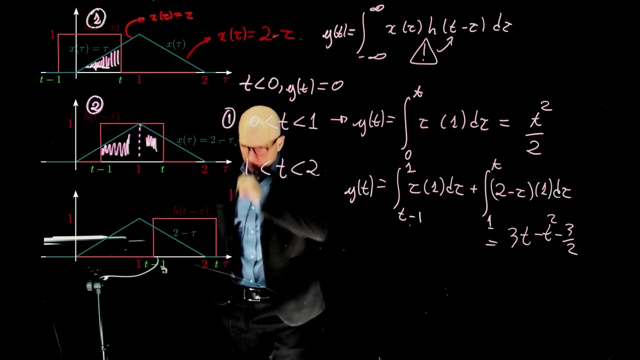 for this result here is: if you do the integration, this is basic math and I guess give the result here: T is three, T minus three, squared plus three and a half. Okay, now we have a very last point here where we passed number two. 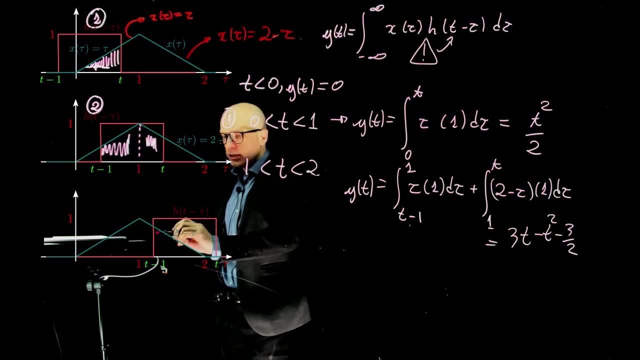 And if you pass number two, see, we are only left with one overlap. This is the only overlap, This is number three as the third region, And this overlap will exist provided that a T is greater than two, because that's where we stopped here.